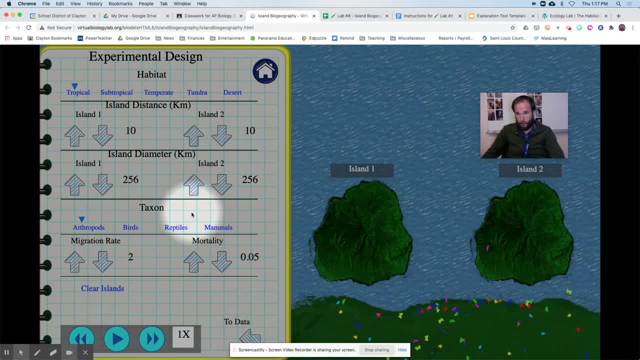 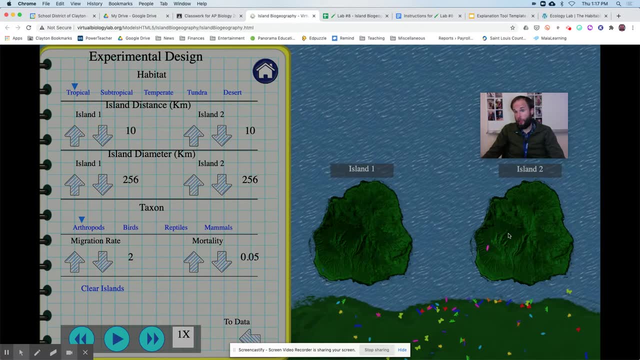 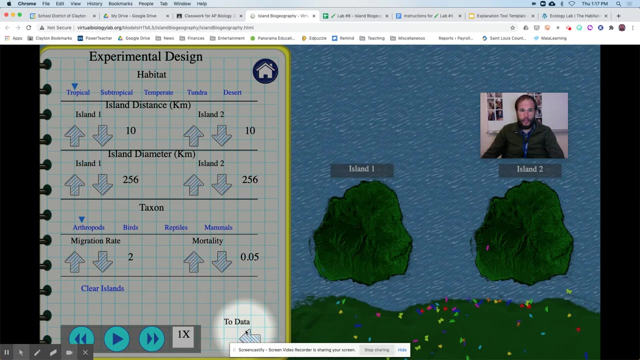 birds, reptiles, mammals. That's just going to highlight the different types of organisms, the different types of species that are either occupying the mainland initially or one or both of the islands later on in the experiment. Okay, but let's hold off on changing the variables right now. Let's go ahead and go back to the data. 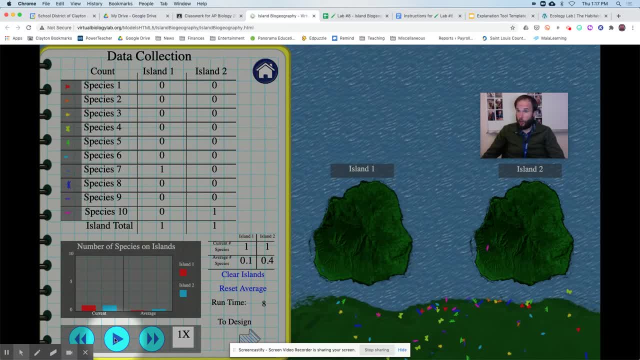 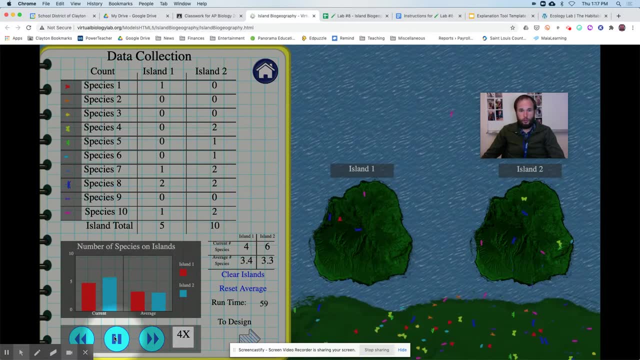 and go ahead and run the simulation under the default conditions. The default setting is kind of slow, so you're welcome to speed it up. What we're going to do is we're going to freeze the simulation at intervals of 100, or as close to 100 as you can possibly get. 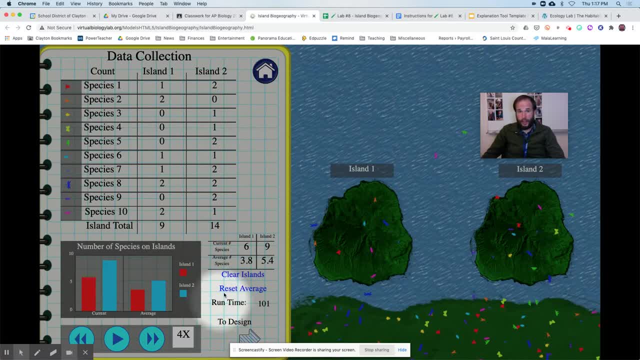 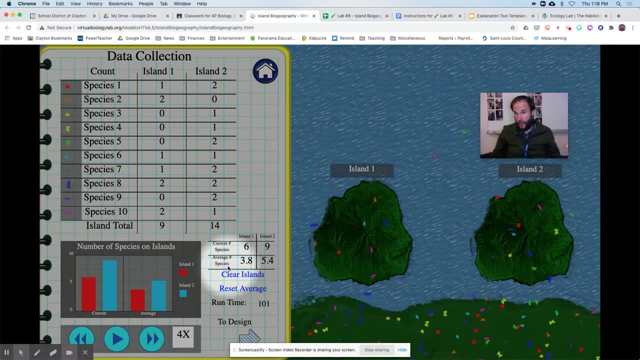 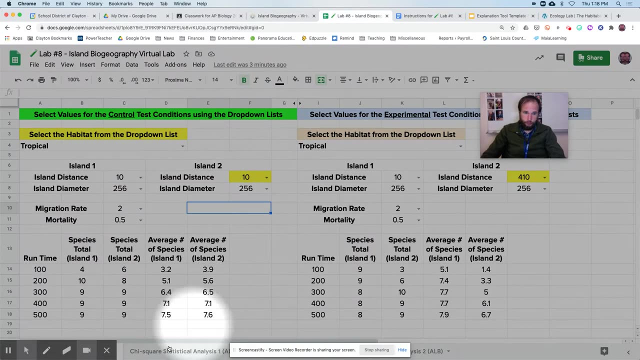 All right. so the data that you're going to be collecting is right here. It's the current number of species on each island, as well as the average number of species over that time interval, In this case, 100 time units. I have shared a spreadsheet with you through Google Classroom: Everything you 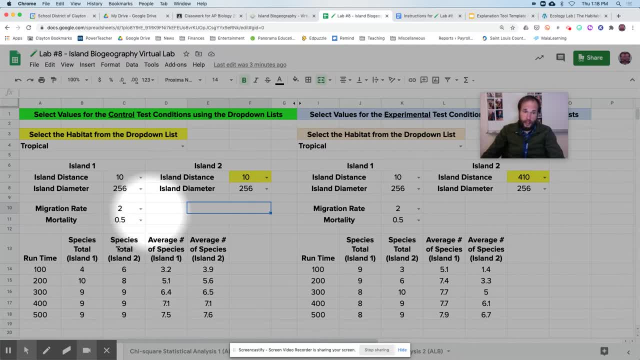 see, here are my sample data, but on the left-hand side of the spreadsheet, this is where you're going to enter your default data. So, again, intervals of 100, and you're going to be recording data at each of those intervals for the total number of species. 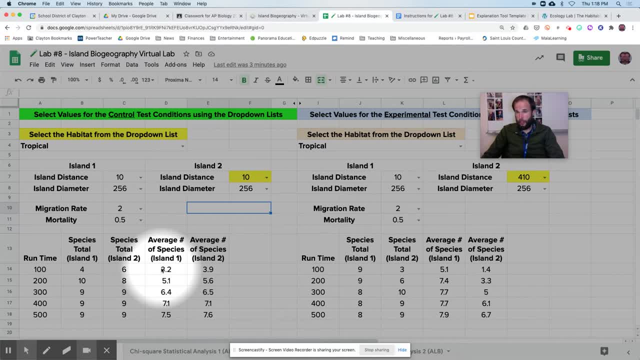 on each island, as well as the average number of species on each island. The rest of these parameters will probably stay the same initially, because they all match the default conditions. Okay, so the goal is to collect data at intervals of 100 for a total time of 500 time units. 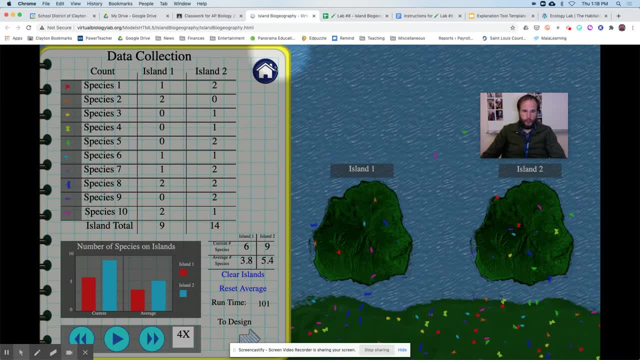 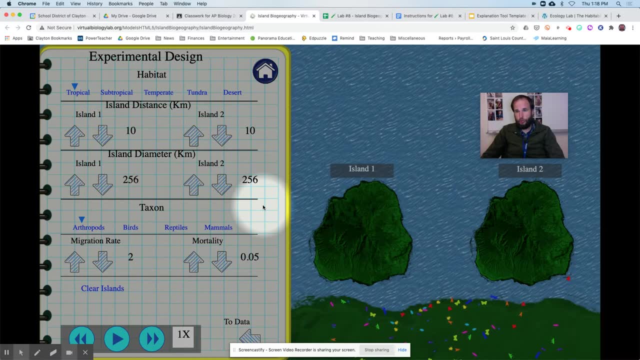 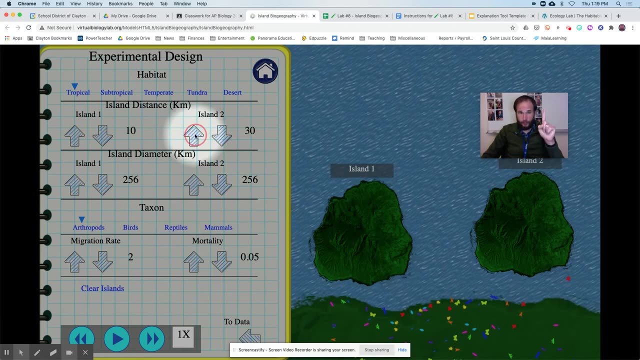 All right, moving on, I'm going to go ahead and reset the entire simulator and this time I'm going to choose a variable to manipulate In the sample spreadsheets that I created. on the first spreadsheet, I manipulated the island distance. I actually moved it as far away as I possibly could. 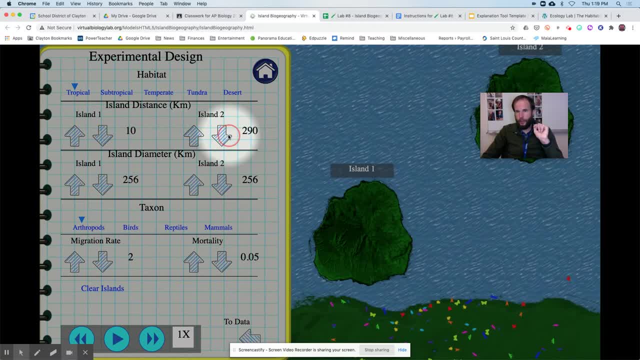 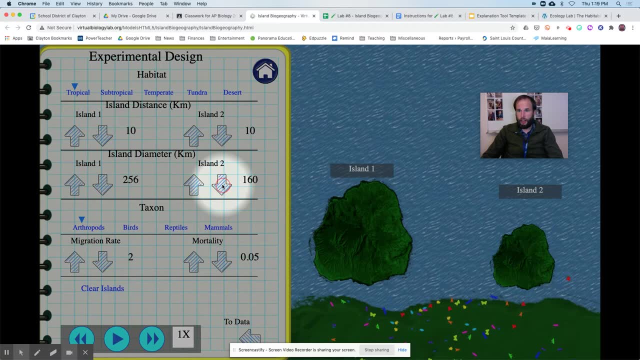 from the mainland. Hopefully, you can see the island moving. For the sake of this example, I'm going to move that island back and manipulate the island diameter. This is the second spreadsheet. second spreadsheet, that sample that I created, and make it as small as I possibly can: 64 kilometers. 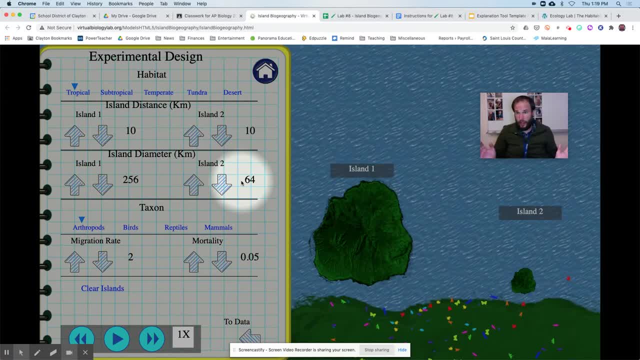 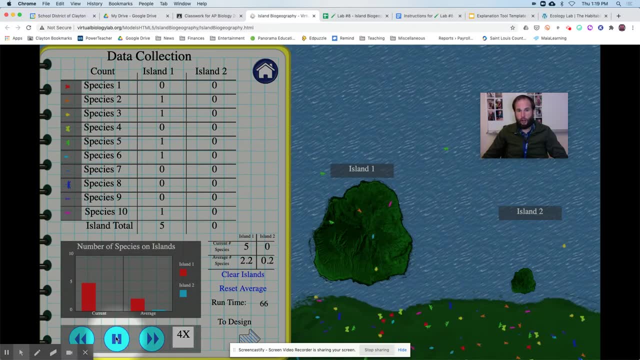 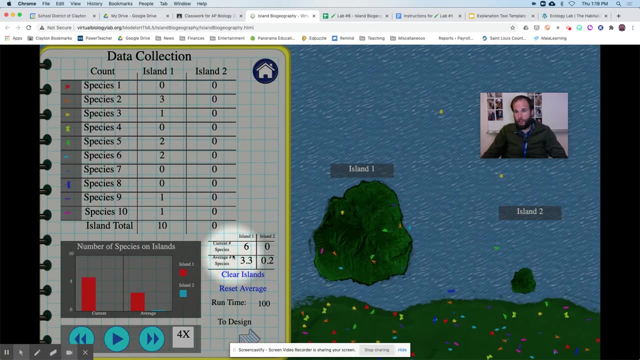 all right, so all of the variables I'm going to keep the same. go back to my data. press start. feel free to speed it up and again at intervals of 100 or as close as you can. you're going to be recording the data and again the data: current number of species on each island, as well as the 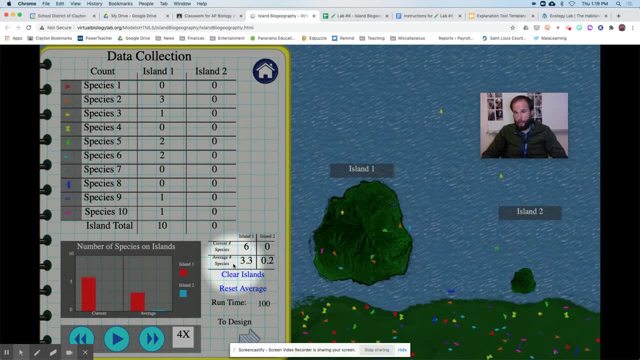 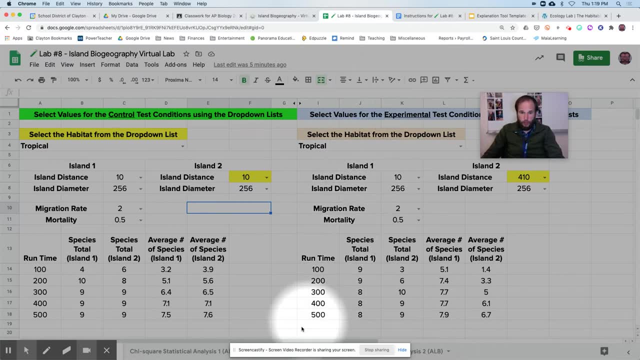 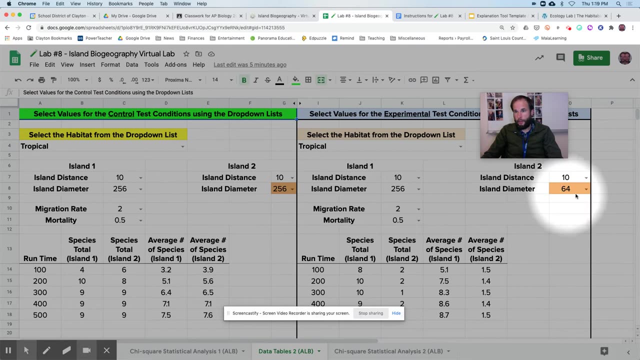 average number of species on each island during that time interval. okay, those data are going to go on the right-hand side of the spreadsheet. okay, in fact, I can show you. here's the second sheet. so there's the island diameter that I changed. this is different from the original. 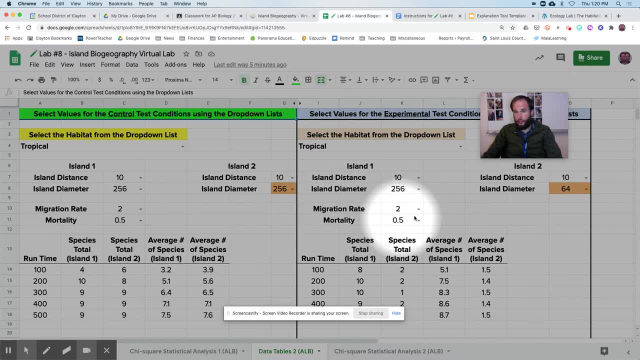 default ion diameter. all the other variables stay the same, and here are my data in the data table. okay, in a row. I'm going to show you how to do that. so I'm going to go ahead and take the values of 100 for a total time of 500 time units. all right, so I have all these data. 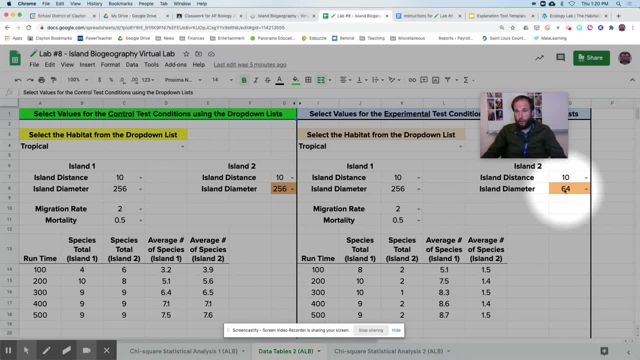 how do I know whether or not changing this particular variable had a significant impact on the number of species that are occupying the island? well, you can probably guess from the sheet down below the title of the sheet down below that we can do a chi-square analysis. now 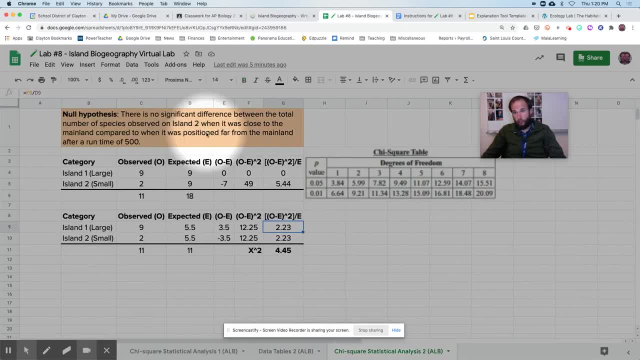 I will say upfront that the null hypothesis that you pose, as well as the analysis that you perform, will be dependent upon the variable that you choose to manipulate. so again, I chose island size when I can already tell, and I'm going to need to edit my null hypothesis because I just 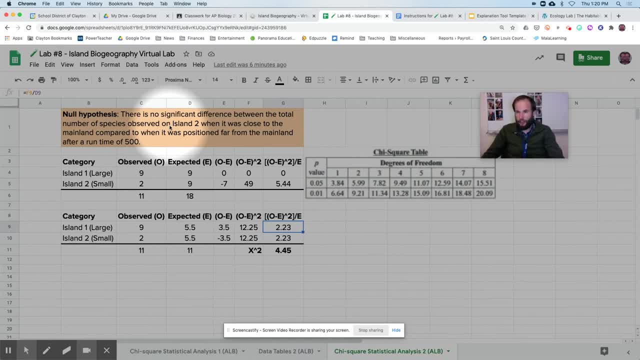 copied and pasted it from the other spreadsheet. that's going to be easy to do. in essence, what I'm going to have to do is revise it to account for the island size and not the island distance from the mainland. but I can tell you that all of the data here where are coming from the previous sheet. 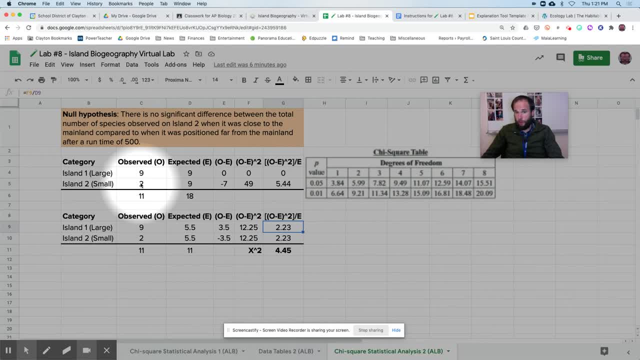 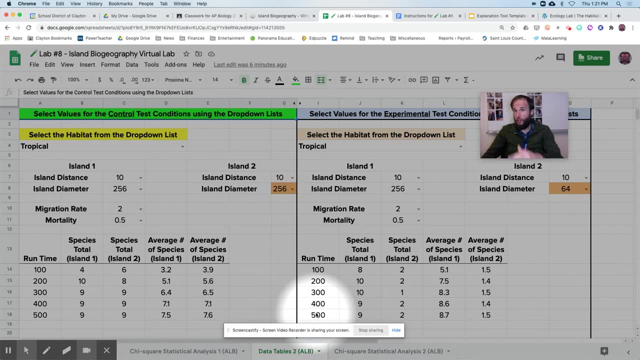 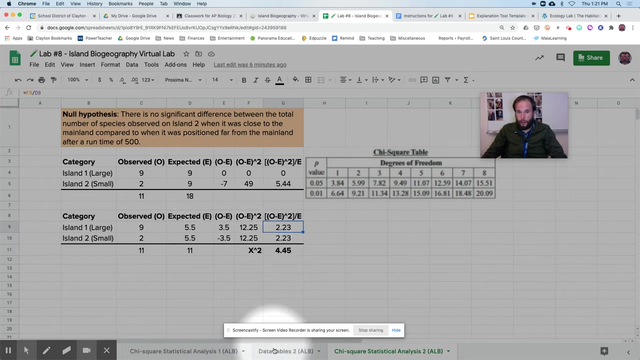 the observed data pretty straightforward. they're coming directly from that 500 time point, right? i want to know how this variable ion diameter changed the species, the total number of species, over the course of time. okay, so those are my observed values, my expected values. well, they're. 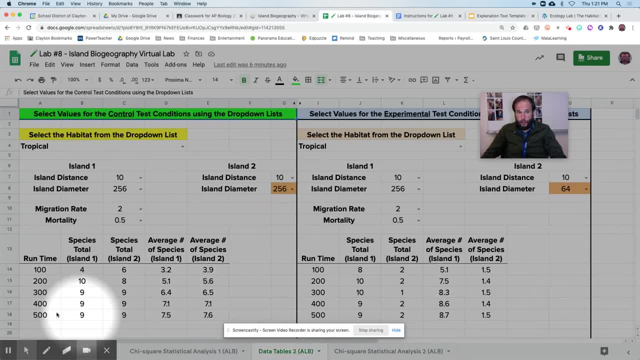 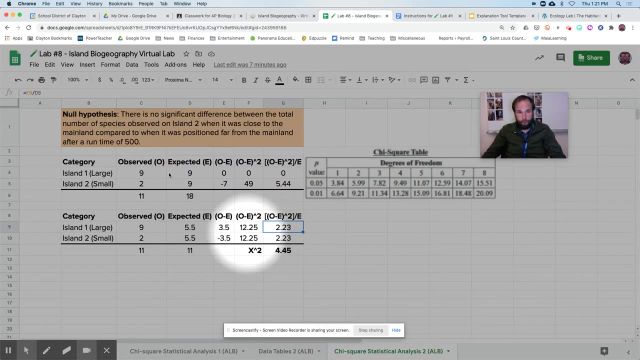 going to come from the control conditions. same time point, remember, the chi-square test is being used to analyze discrete data, but this time i want to know what the species diversity would have been had i never changed the island size. okay, so when i go back to this sheet right, i'm comparing. 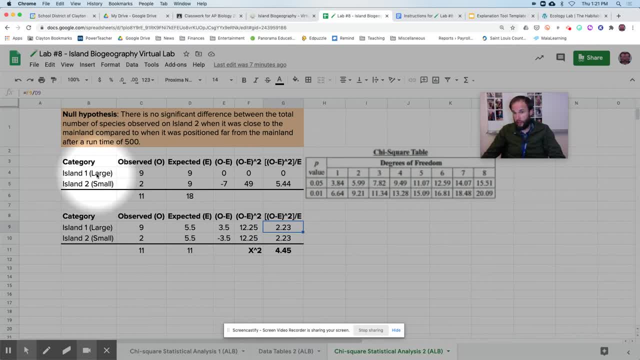 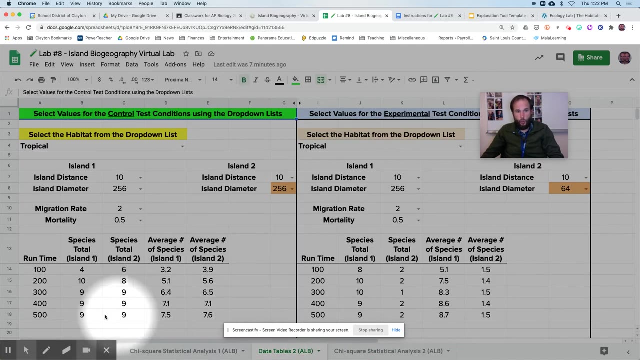 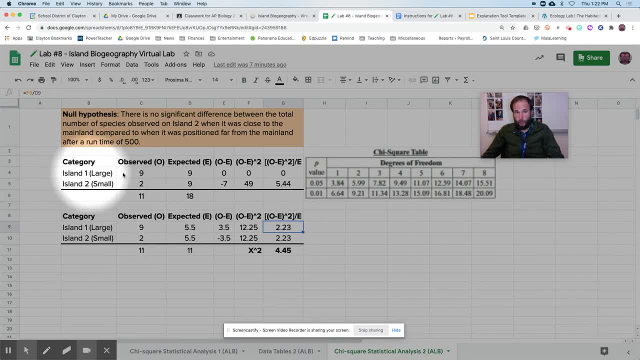 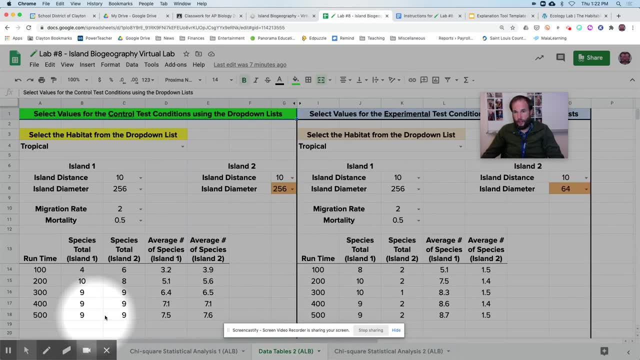 island one. right, it's also nine. I go back. you can see that over here again. I'm using for my expected conditions right from expected values under the default condition conditions after 500 time units. I expect both island 1 and island 2 to have 9 total species. 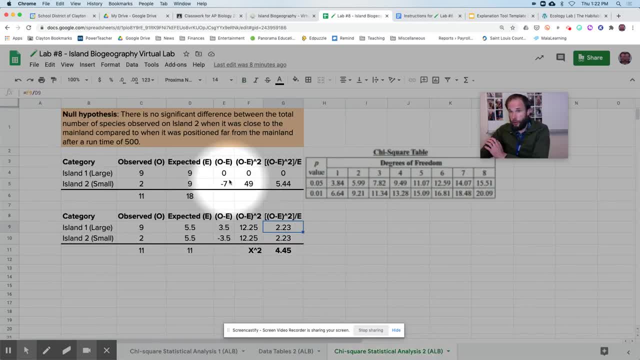 Alright. Well, what you run into if you enter those values is that the observed total does not equal the expected total. So I have to manipulate my data a little bit to make those two sums equal to each other, But it's pretty easy to do. 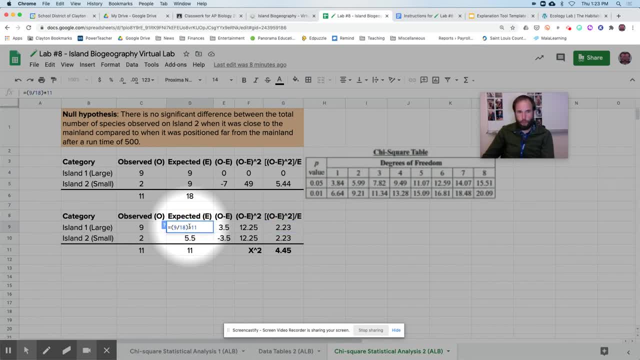 Down here. I've actually done that work for you, So I had an expected value of 9 here. There were 18 total observations that I made, So that fraction times 11, which is the sum of the number of observed values, observed species, that formula 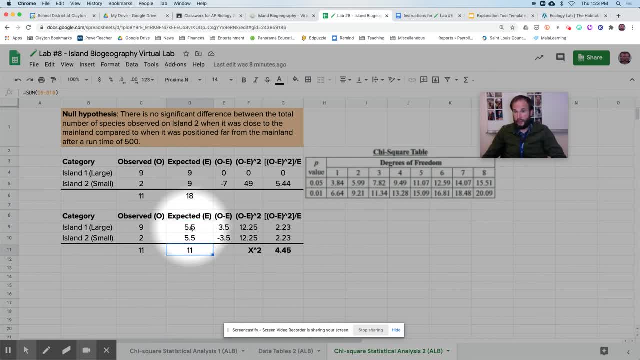 will kind of transform the expected value in a way, so that when I sum those two values together, now the number of observations for both of those two groups, the observed and expected groups, they equal each other. If I left the data as I did up here, I'd be comparing. 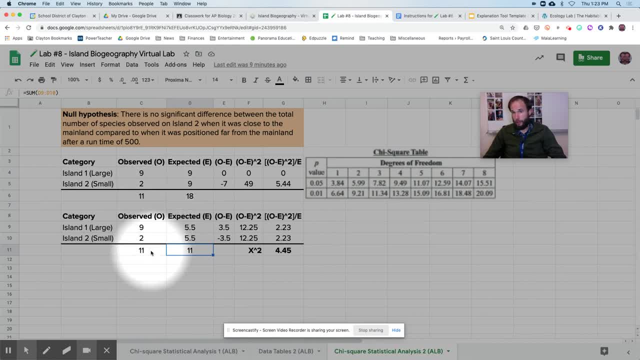 apples to kumquats. That's not going to work. Here I'm comparing Macintosh apples to Granny Smith apples. So I go ahead and do the chi-square analysis, I get my chi-square statistic And I'm going to compare that to my critical value. Well, the way that I set up this, 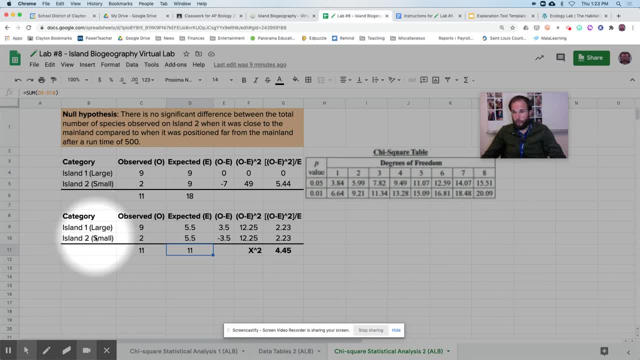 analysis. I had two different groups, two different islands, So I've got two categories. That's a one degree of freedom. It's always safe to use my p-value of 0.05, that 5% chance, that 5% probability that the difference between the two groups is.